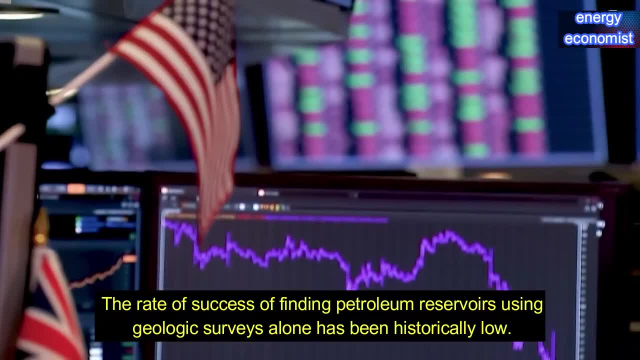 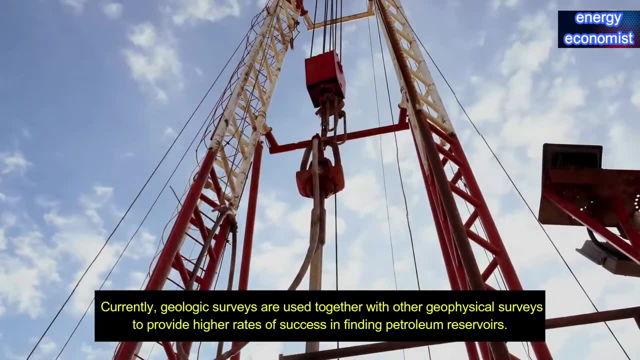 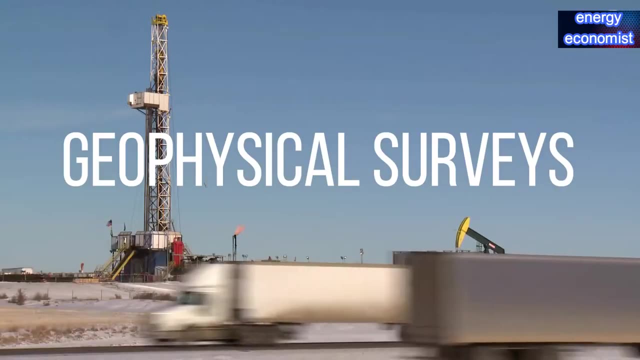 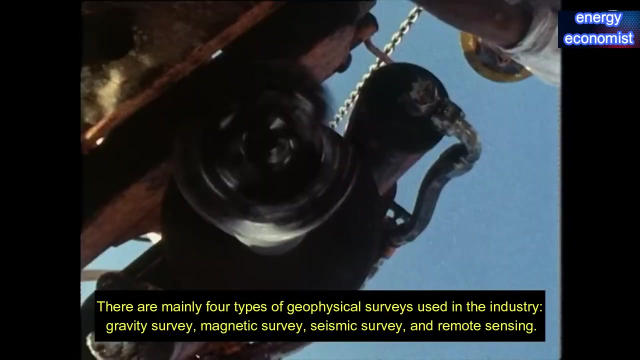 geologic surveys alone has been historically low. Currently, geologic surveys are used together with other geophysical surveys to provide higher rates of success in finding petroleum reservoirs. Geophysical surveys: There are mainly four types of geophysical surveys used in the industry: gravity survey. 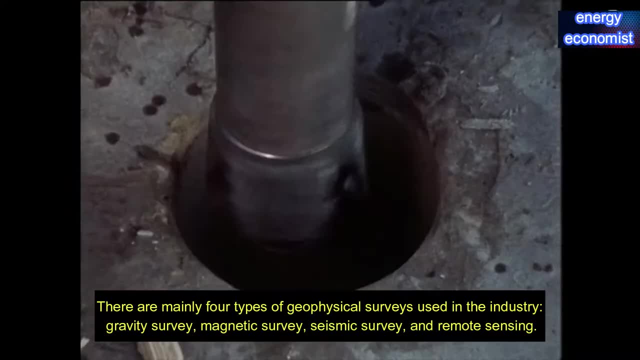 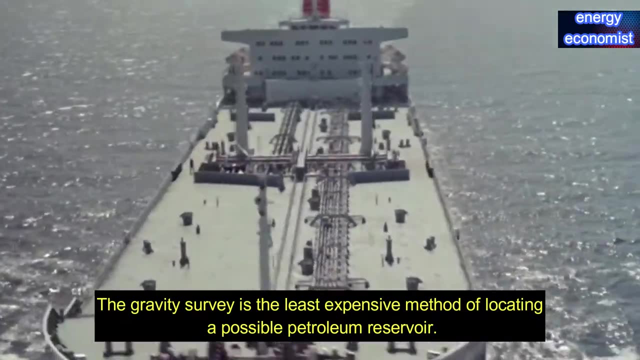 magnetic survey, seismic survey and remote sensing. The gravity survey is the least expensive method of locating a possible petroleum reservoir. It involves the use of an instrument, a gravimeter, which picks up a reflection of the depth of the reservoir. The gravity survey is the 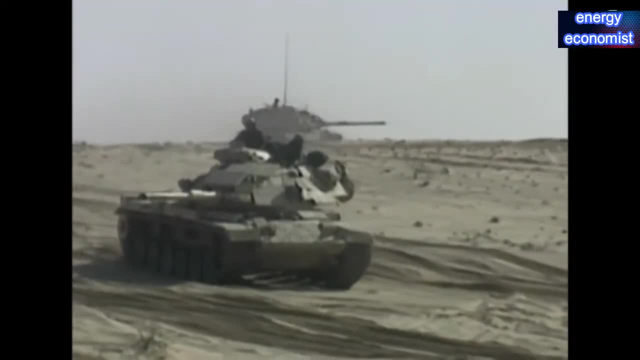 most expensive method of locating a possible petroleum reservoir. It involves the use of an instrument, a gravimeter, which picks up a reflection of the depth of the reservoir keynote The magnitude of long can認知 salt density of the surface rock, For example. because 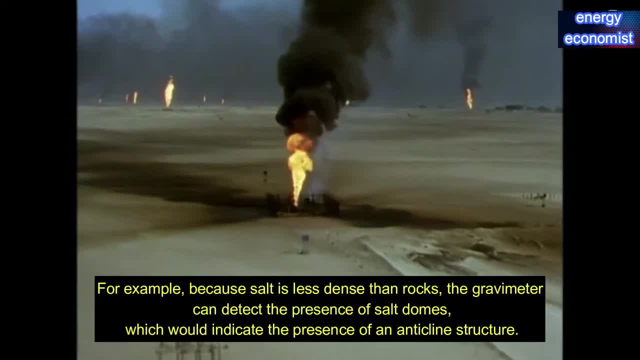 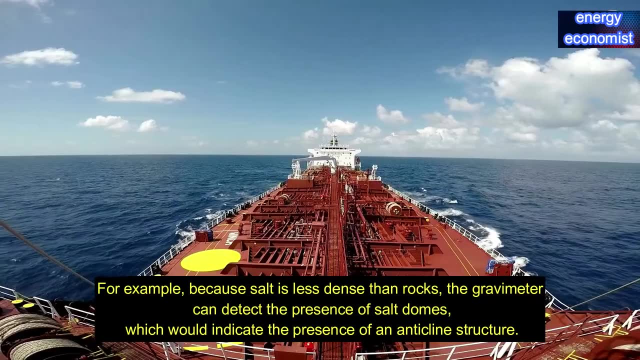 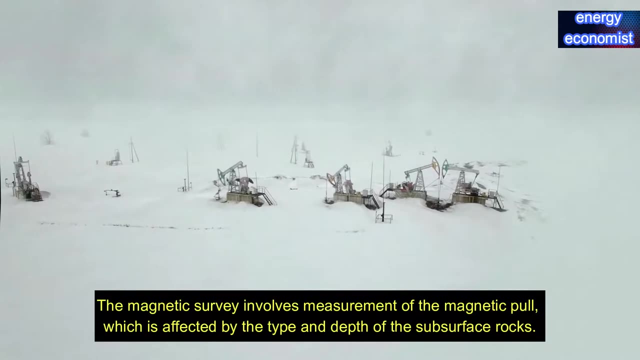 salt is less dense than rocks. the gravimeter can detect the presence of salt domes, which would indicate the presence of an anteclay structure. Such a structure is a candidate for possible accumulation of oil and gas. The magnetic survey involves measurement of the magnetic pole which is affected by the type and depth of the subsurface rocks. 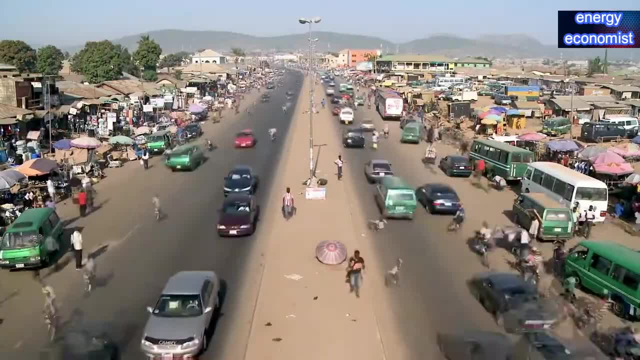 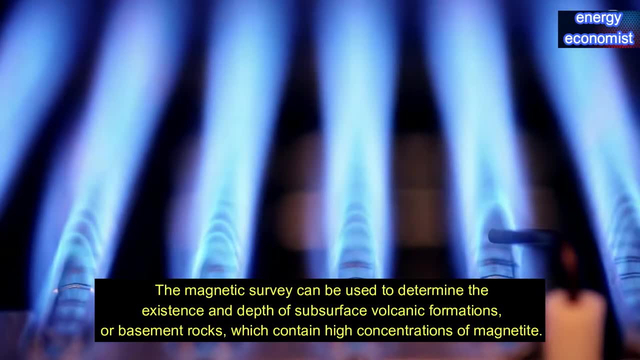 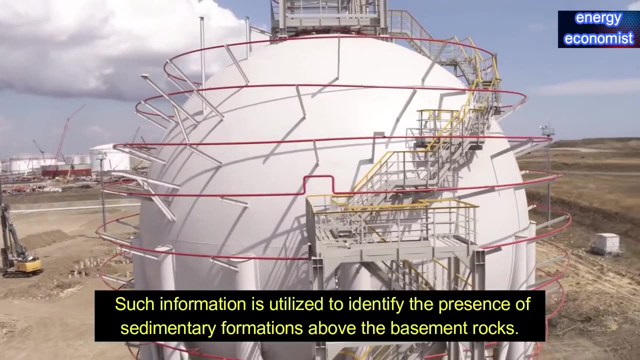 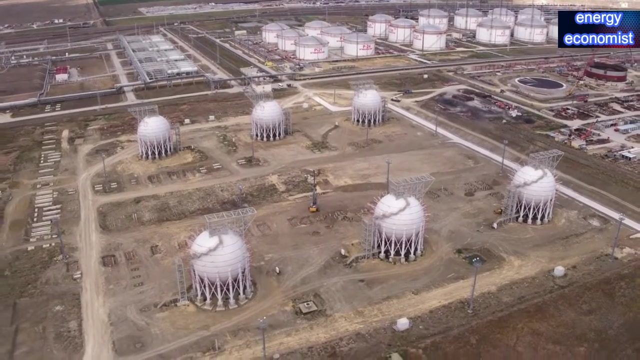 ity. The seismic survey can be used to determine the existence and depth of subsurface volcanic formations or basement rocks which contain high concentrations of magnetite. Such information is utilized to identify the presence of sedimentary formations above the basement rocks. The seismic survey involves sending strong pressure through the earth and receiving 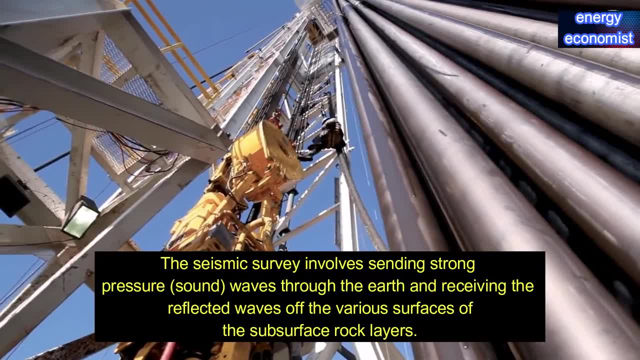 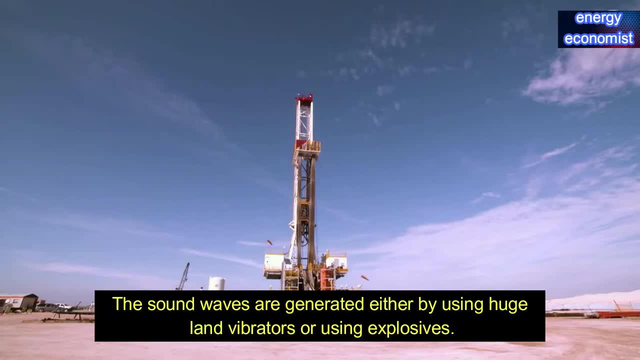 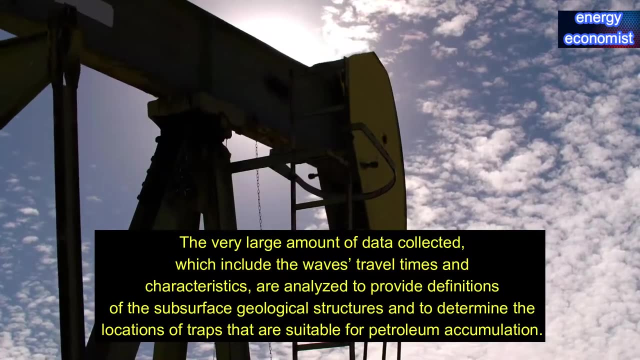 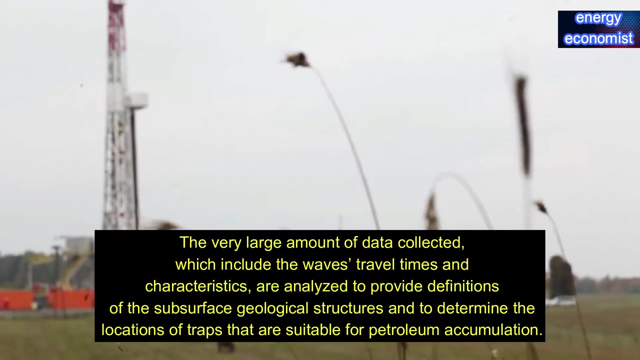 the reflected waves of the various surfaces of the subsurface rock layers. The sound waves are generated either by using huge land vibrators or using explosives. The very large amount of data collected, which includes the waves, travel times and characteristics, are analyzed to provide definitions of the subsurface geological structures and to determine.